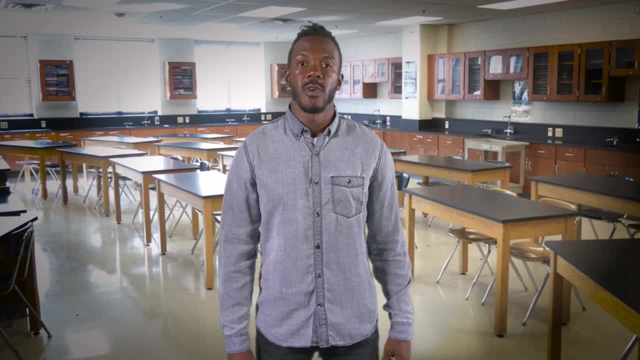 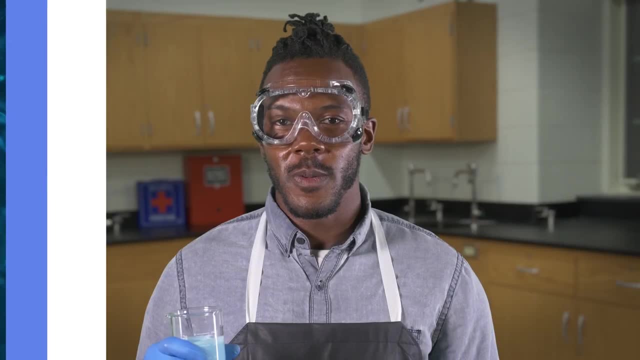 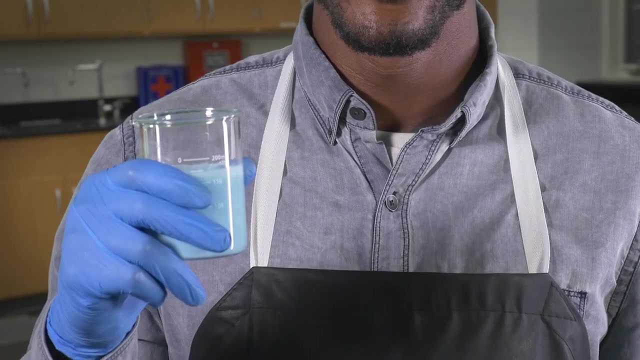 can easily become entangled in equipment or be exposed to hazardous chemicals. When exposed to flames, hair can even catch on fire. Let's run a little experiment. Imagine for a moment you're in the lab and your lab mate accidentally jostles your arm while you're holding a beaker or test tube filled with. 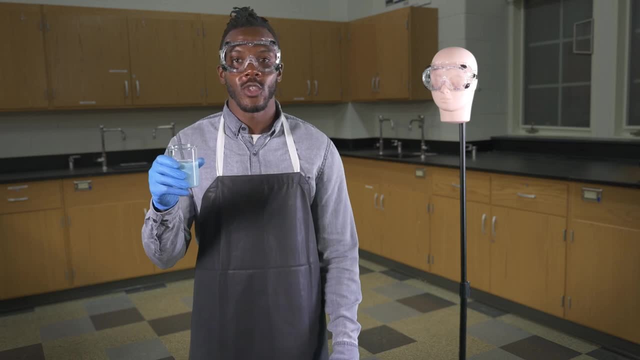 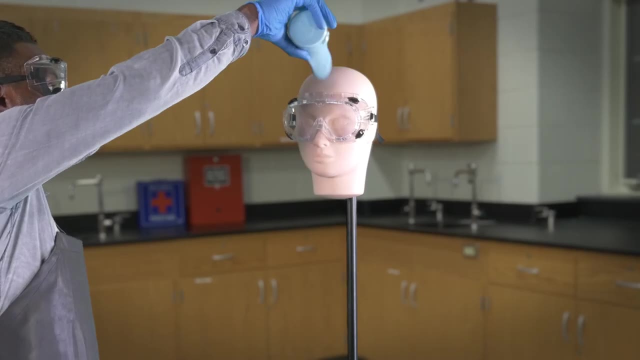 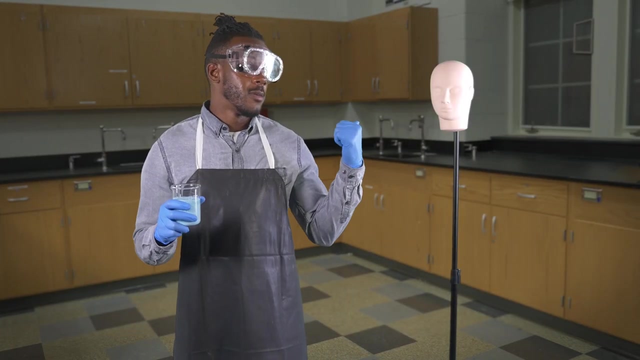 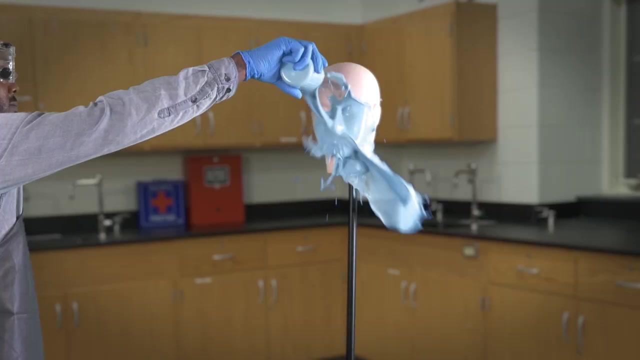 liquid. What's the worst that could happen? If you're wearing eye protection, like test dummy one here, it might look something like this. And if you don't wear eye protection in the lab- like dummy number two- something you would never do, right, It looks something like this. 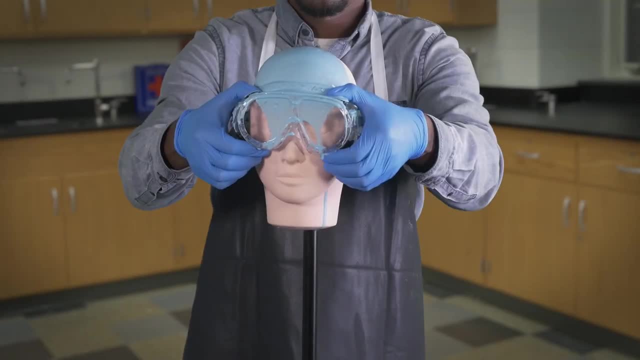 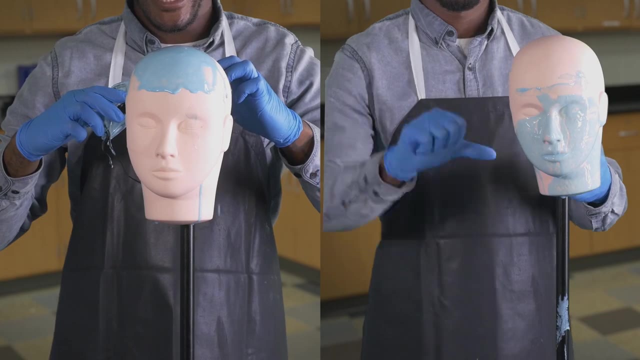 Now let's do a side by side comparison. As you can see, the eyes of dummy one were protected from the liquid by splash goggles. Dummy two, on the other hand, didn't fare so well In this demonstration. the liquid was just buttermilk with some food coloring added to it. But imagine. 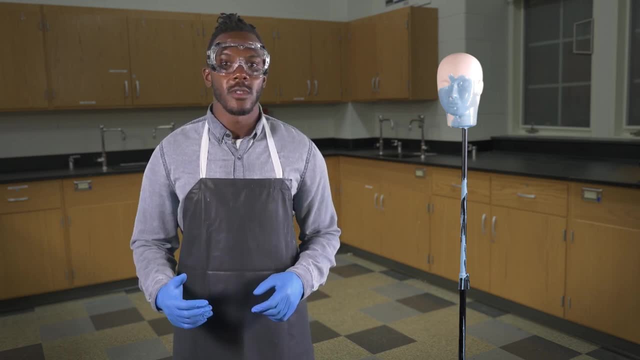 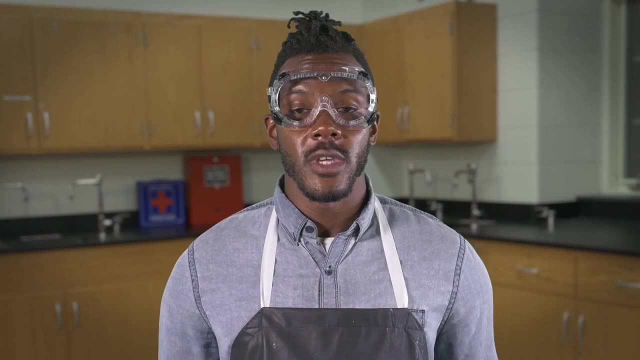 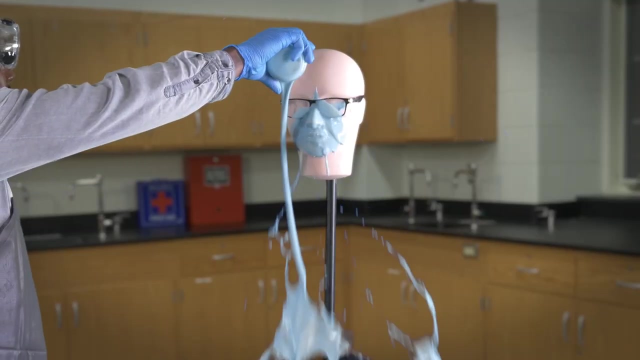 your head gets splashed with hydrochloric acid, a highly corrosive substance. It'd be a much grimmer picture for your poor eyes. Now, if you wear prescription glasses, you might be thinking: maybe these will protect me. There's only one way to find out. 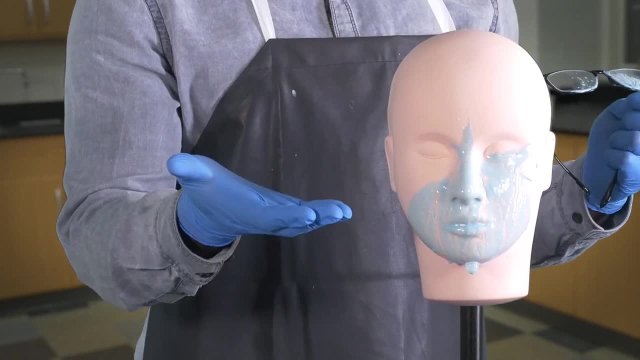 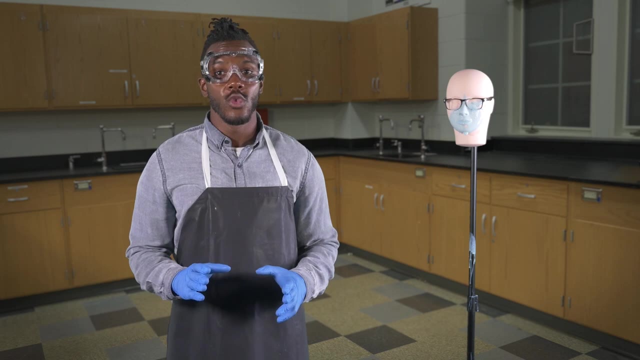 As you can see, eyeglasses are better than nothing, but not as good as goggles. Prescription glasses are required to meet standards for impact resistance, but they won't protect you from splashes or liquids dripping behind your glasses. Then there are typical safety. 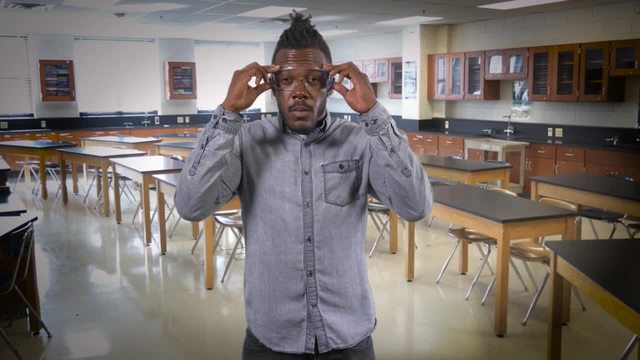 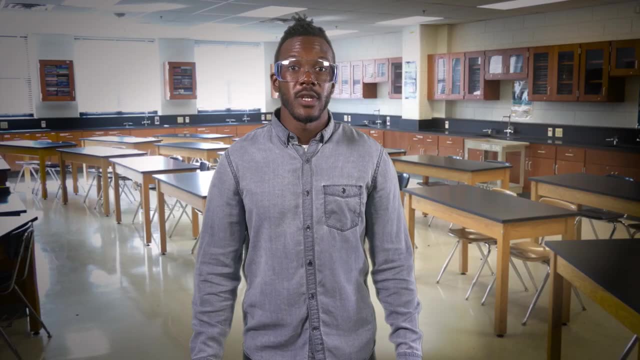 glasses used in places like construction sites. These are a bit better because they often have a splash guard above the lenses. The problem is the guard doesn't conform to the face, so there isn't any real protection against splashes, Only chemical splash goggles usually. 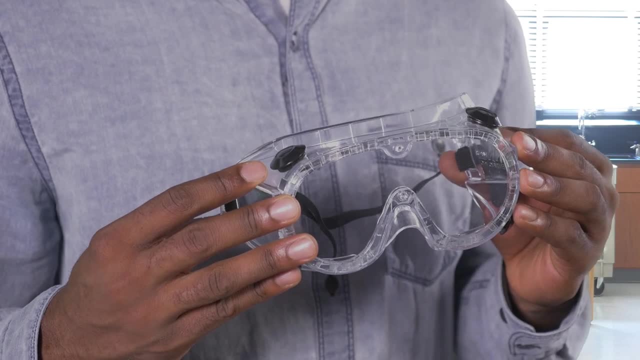 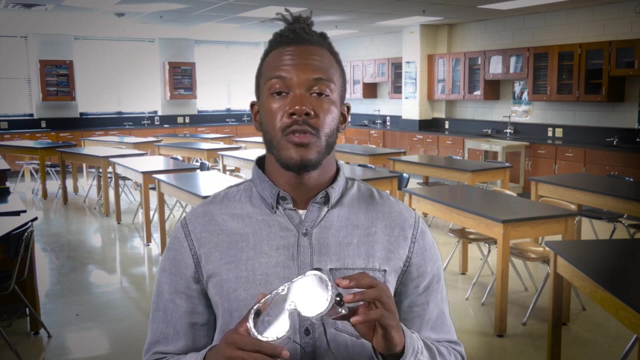 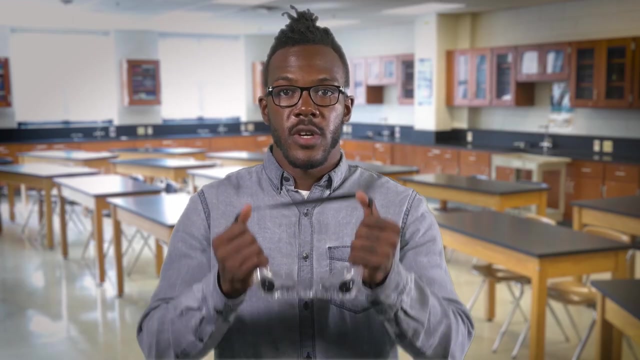 just called safety goggles provide full splash and impact protection for the eyes. Safety goggles come in several sizes and colors. Adjustable elastic straps allow them to be fitted closely to the face. They're also vented, and these venting plugs should never be removed. Chemical splash goggles are designed to fit comfortably over prescription glasses. 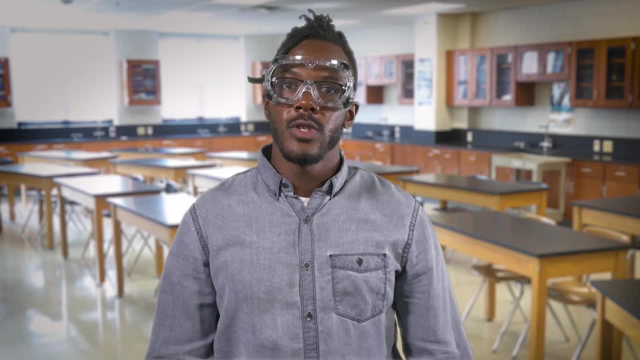 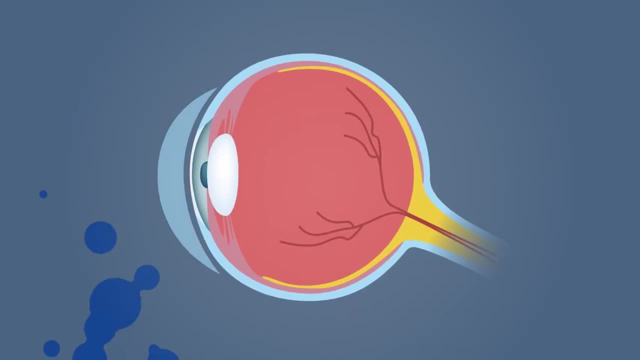 and must always be worn with contact lenses as well, to minimize the risk of getting chemicals in your eyes. If you wear soft contact lenses, you should be aware they can absorb chemical vapors that pass through the vents of the safety goggles, In this case your teacher. 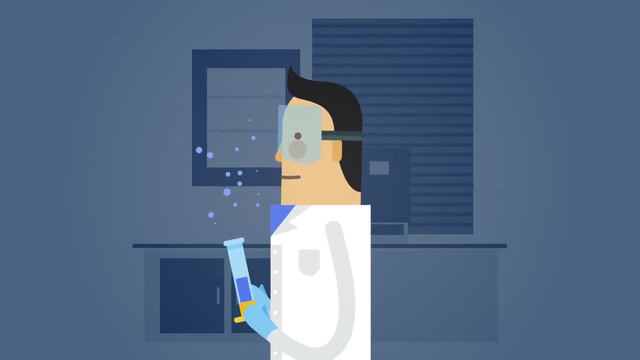 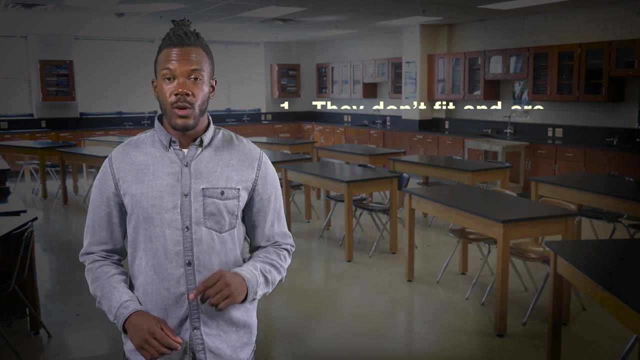 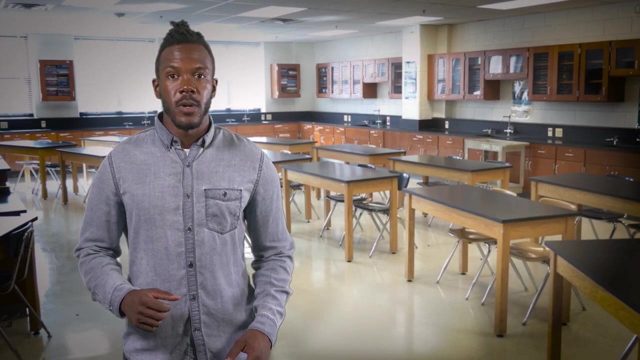 may recommend wearing special, un-vented goggles. Let's be honest: We know many students don't like wearing safety goggles and we hear two main complaints: One, the goggles don't fit and are uncomfortable, and two, they fog up. The first step in getting goggles to fit comfortably is to pick an appropriate size for your face. 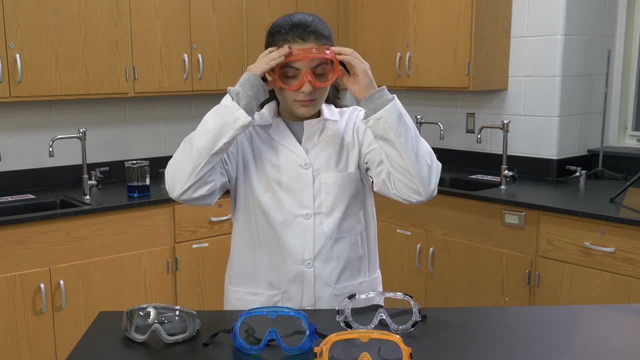 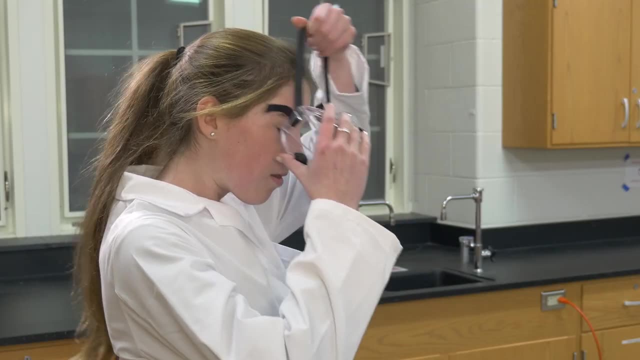 If you have problems with the way the goggles fit, ask your teacher for a smaller or larger size, And once you're in the ballpark you can adjust the fit by tightening or loosening the elastic strap. The goggles should fit snugly, but they shouldn't cut into your cheeks If you see deep marks. 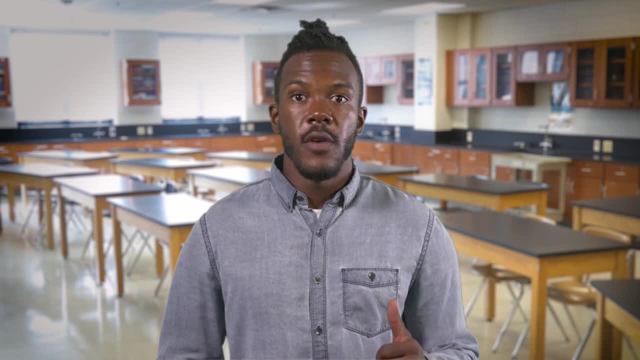 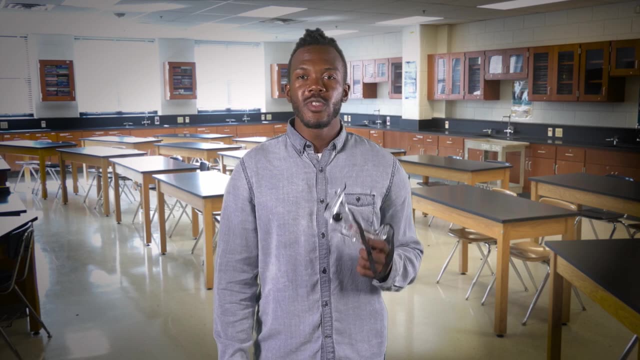 on your face after they're removed. the goggles are too snug. If they move around too freely, they're too loose. The other common complaint is that goggles fog up when worn. Here's a quick snowboarder's trick that may help Rub a little soap solution on the inside of the lenses to avoid fogging. 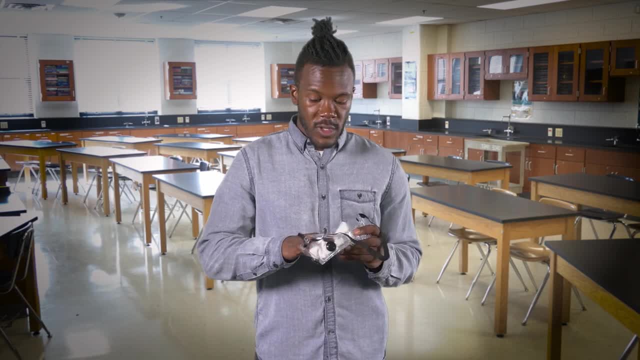 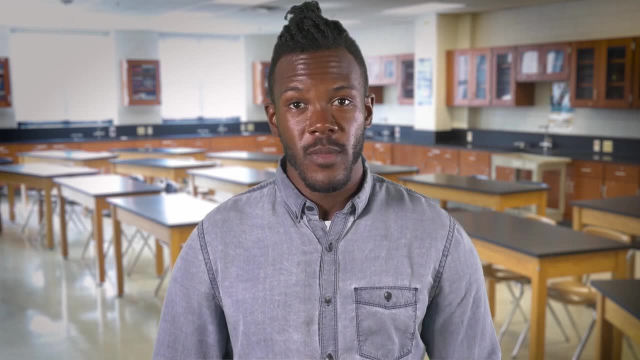 Just be sure to polish the lenses dry before putting on the goggles. Look, almost every sport requires you to wear some kind of protective gear. You should always wear a protective protection. The same is true for the lab. Wearing the appropriate PPE is essential. 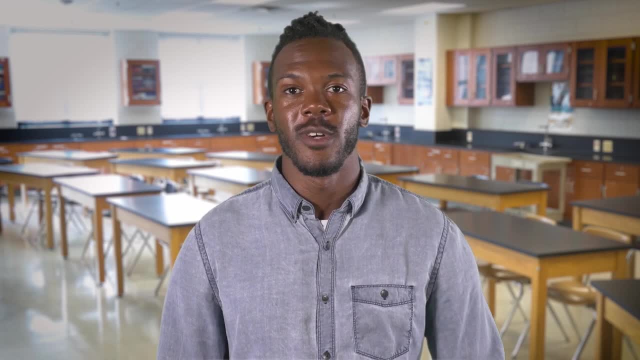 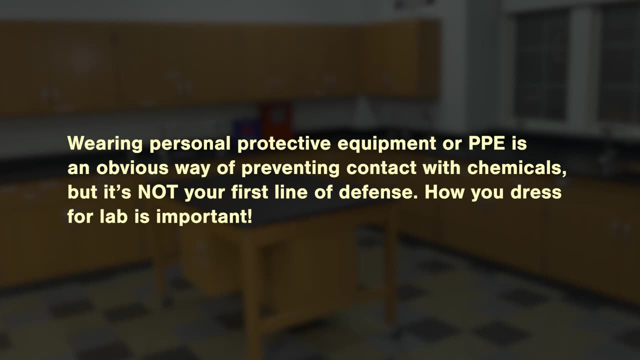 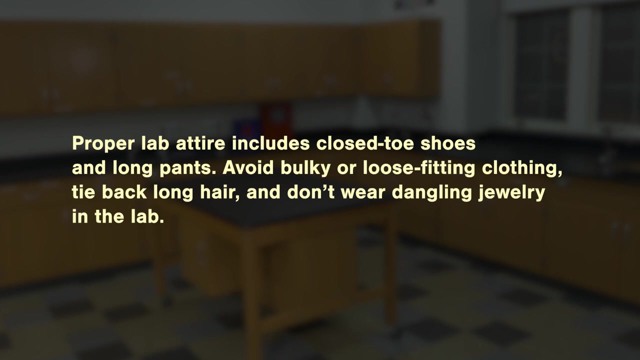 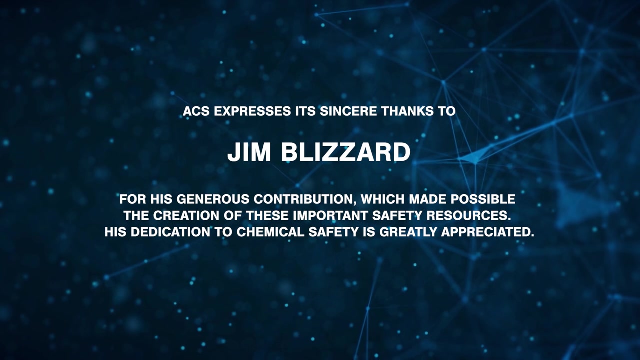 for all lab activities. so be sure to suit up with the correct gear. Apply a potent softener to the tablecloth, greatly reorganized for. prevent curdling and이드 preemptively. Your goggles really should not heighten, even after 195 percent. 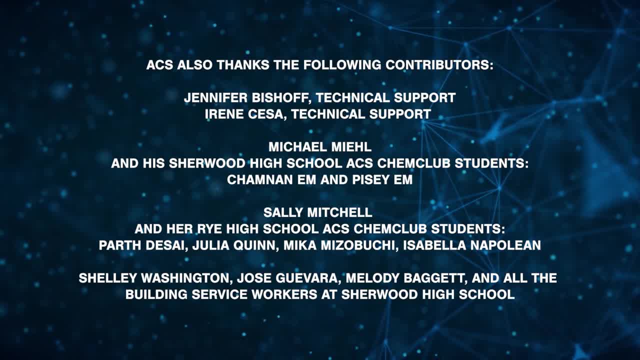 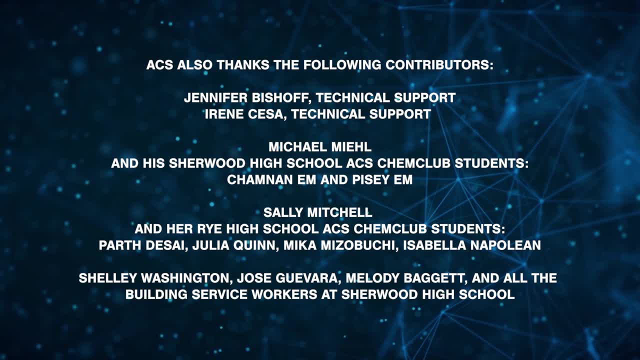 If you decide to wear them raw, make sure they are perfectly covered with protective protection. again, musimyid At least 4 times a day. choose a heavyweight—a winter iceAT— dinero 3 times heavyweight figure, First-Namely, with double-足 boiling water.